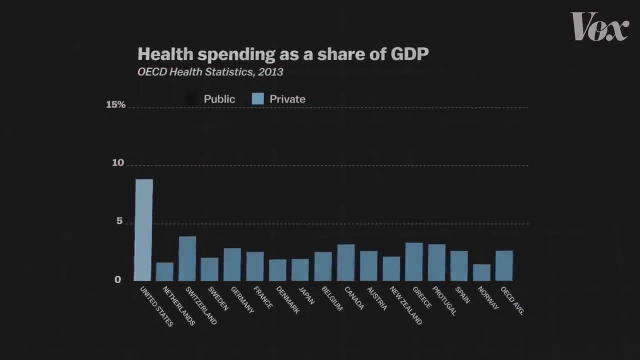 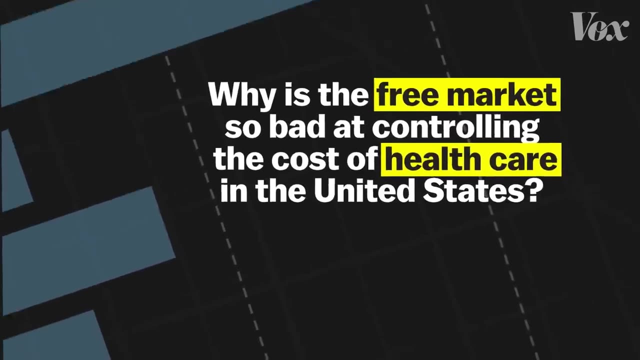 Give it to the private sector. That is what we hear in America all the time, And yet here we are, with the biggest private sector spending the most. Why is a free market so bad at controlling the cost of healthcare in the United States, If you look at the data on physician visits and 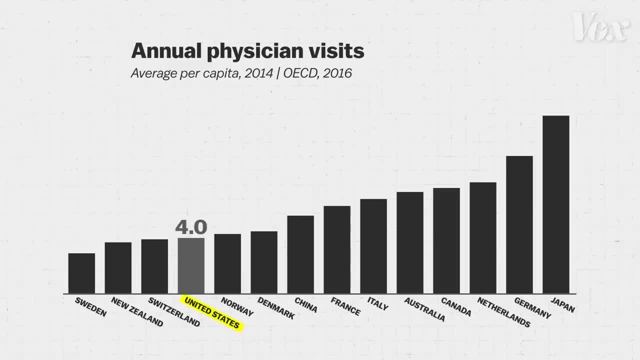 hospital discharges, you can get rid of one theory: Americans don't consume more healthcare than people in these other countries. We don't go to the doctor more than the Germans or the Japanese. In fact, we go to the doctor less. The difference between us and them is that we pay more. 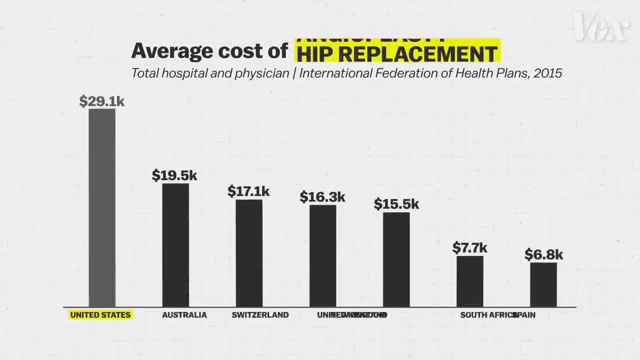 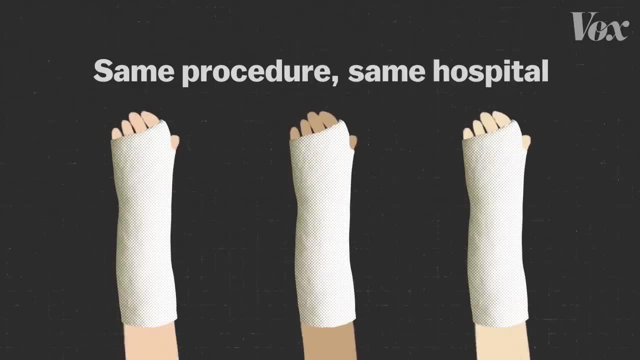 every time we go to the doctor for everything from an angioplasty to a hip replacement, from a C-section to a pain reliever. In America, the price for the same procedure at the same hospital. it varies enormously depending on who is footing the bill. The price for someone with public insurance like Medicare or Medicaid is often the lowest price. These groups- they cover so many people that the government can demand lower prices from hospitals and doctors and they get those lower prices. If the doctors and hospitals say no, they lose a ton of business. 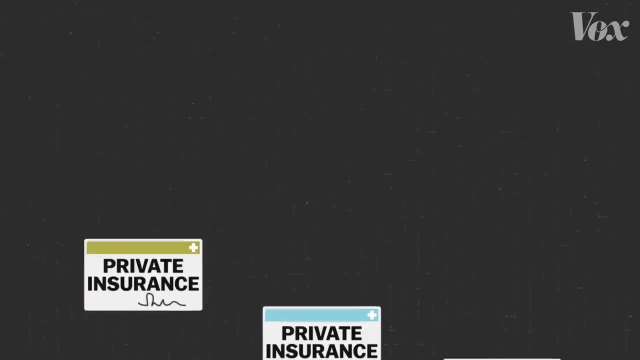 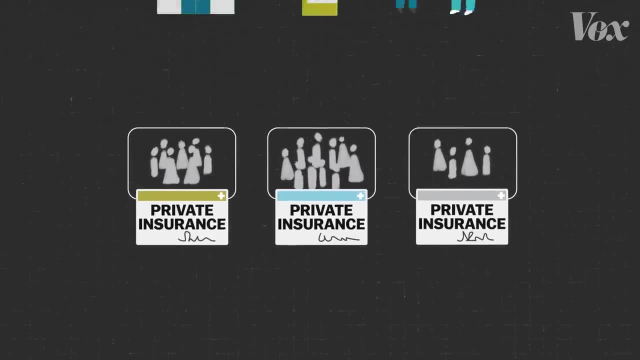 They lose all those people on Medicare, all those people on Medicaid. But there are hundreds of private insurance companies and they each cover far fewer people than a Medicare or a Medicaid, And each one has to negotiate prices with hospitals and doctors on their own. And if you're uninsured, you have even less leverage. Nobody is negotiating on your behalf, So you end up paying the highest price. One study found that most hospitals charge uninsured patients four times as much as Medicare patients for an ER visit. Other countries they don't have this problem. 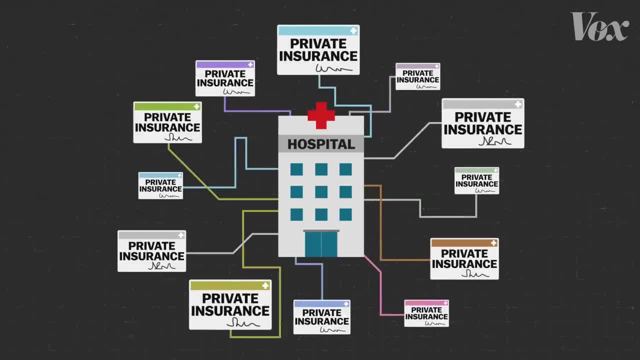 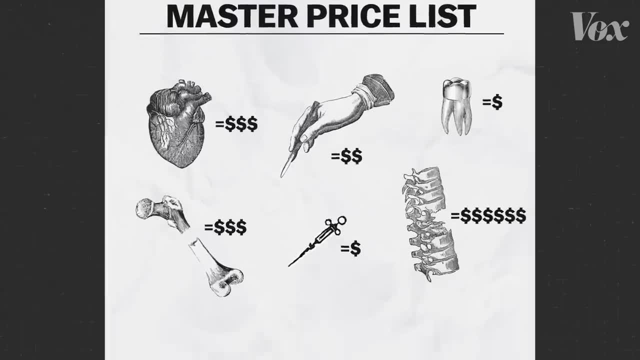 Instead of every private insurance company that has insured patients. they charge private insurance company negotiating with every healthcare provider. there's just this big list country, the central government. they go and they say: if you want to sell to us, to all of our people, then here is what you can charge for a checkup. here's what you can charge for an mri or a prescription for. 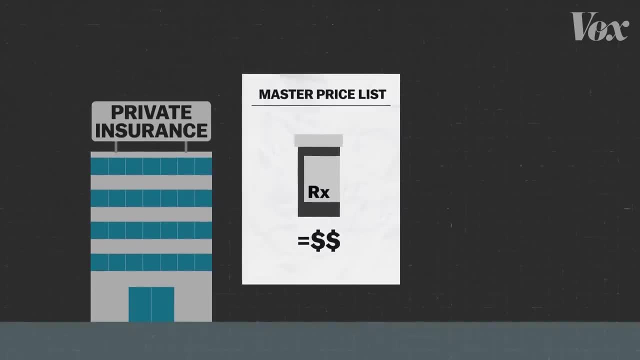 lipitor. and so then, whether that bill goes to the heavily regulated private insurance companies in germany or directly to the government, like in the uk, each country is telling the doctor or hospital or drug company how much that bill will be, and because the government controls access to all of 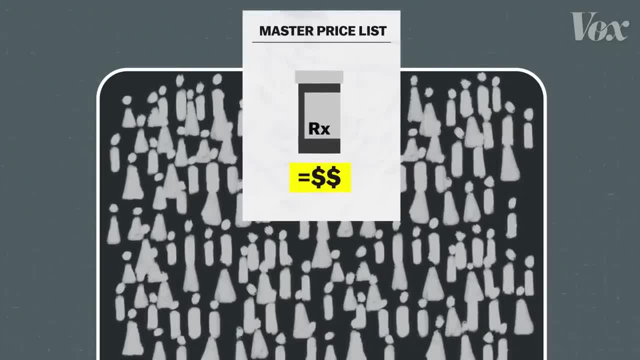 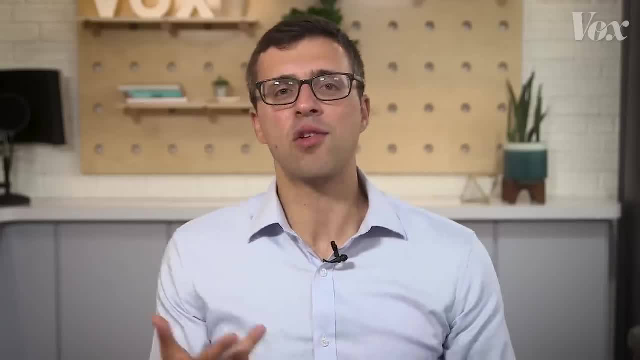 the customers. it's an offer that hospitals and doctors and pharmaceutical companies typically can't refuse. i'm gonna make him an offer he can't refuse in america. the idea is that you'll be a consumer, that you'll do what you do when you go to best buy and buy a television, but that just. doesn't work in healthcare. it doesn't work in healthcare because you often come get healthcare when you're unconscious in an ambulance, when you're scared, when it's for your spouse or your child. it is a time when you have the least bargaining power. you are not usually capable. 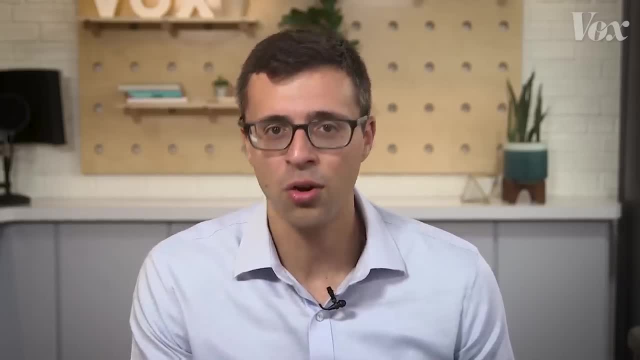 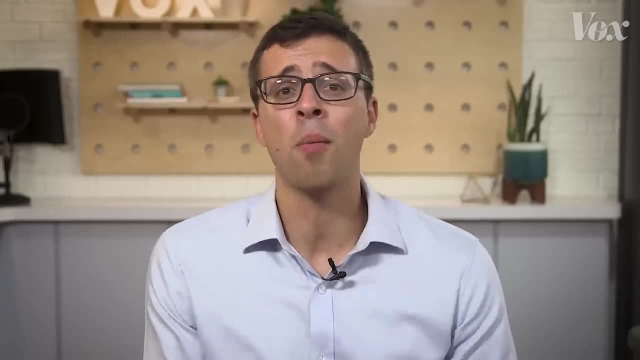 of saying no, you're not knowledgeable enough to do it, you're not comfortable doing it or you're not conscious enough to do it. that's why, in other countries, the government is a person who can say no for you, who can say no, that's too expensive, you're gonna have to lower your price because they do have that power. 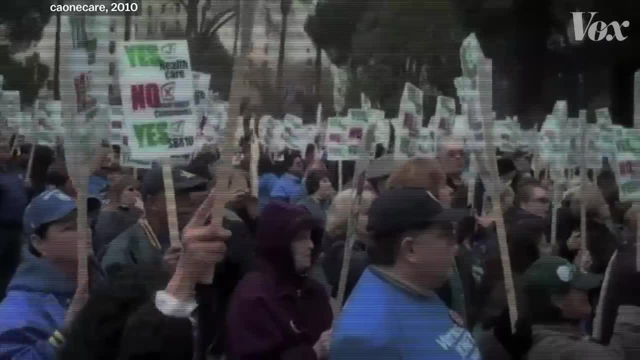 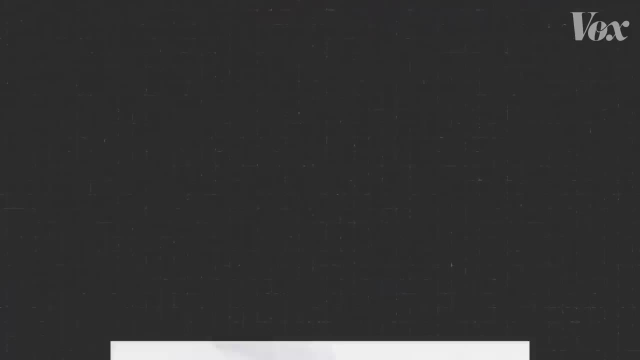 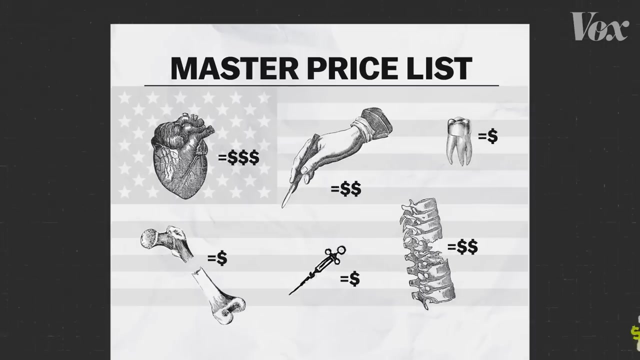 a new push for single-payer healthcare. right here in the us, california and others are saying maybe we should adopt the european model. if we decided to create a single-payer system with one of these huge priceless in the us, there'd be nothing to stop lobbying from hospitals, from doctors, from drug companies and those prices would get. 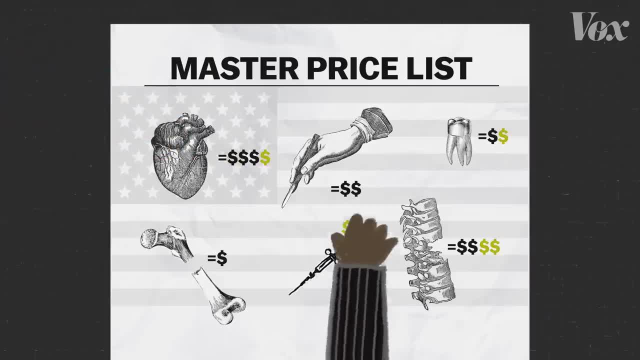 influenced, so we could end up with a single-payer system that is expensive, even as expensive as our current system. it all depends on how much you negotiate down the prices, and now in america these groups have so much power, because they are so rich, that it's really hard to get them. 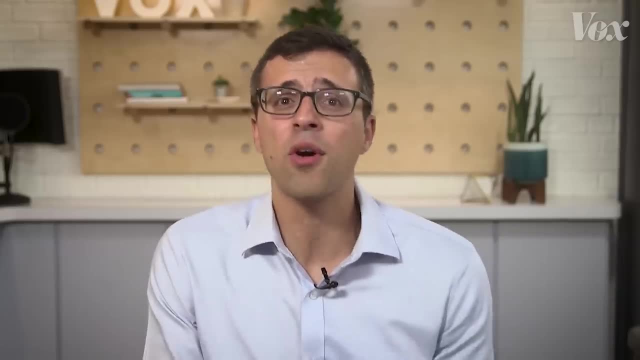 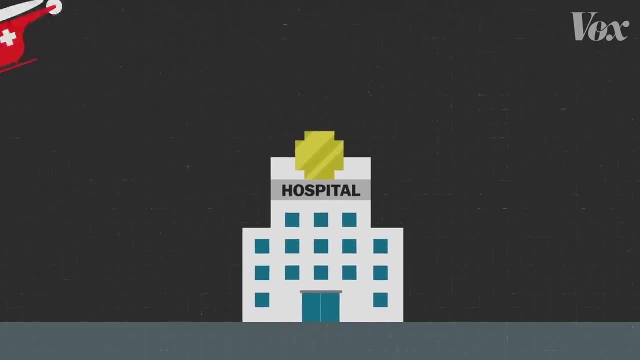 to bring down the prices. this is the irony of american healthcare: it's so expensive that it's become hard to make it cheaper. all that money they make, that becomes political power in years and years and years of over. Democrats, you're talking about the power of media, because 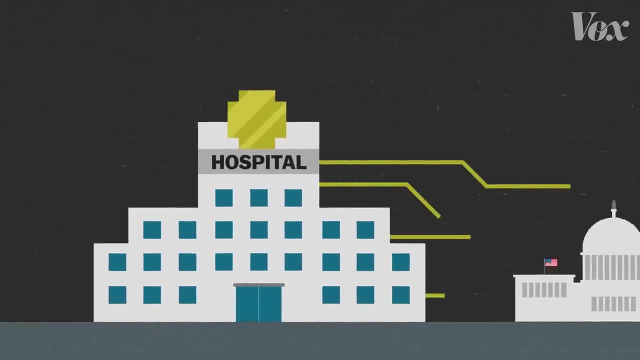 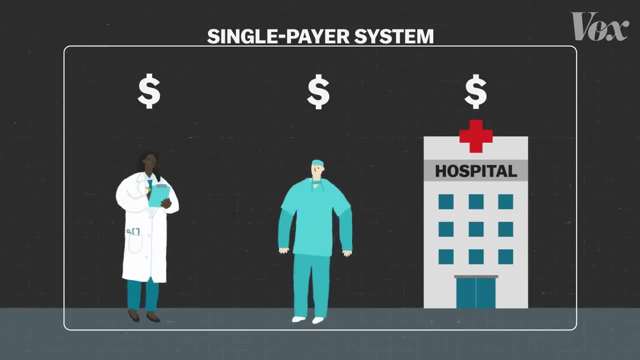 that's what governments do w hottest ones do laws that measure how much money they make, but when you, we're paying. Those are huge industries now and they have a lot of influence in Congress Under a single payer system. if we did drive prices down- doctors and hospitals, they would 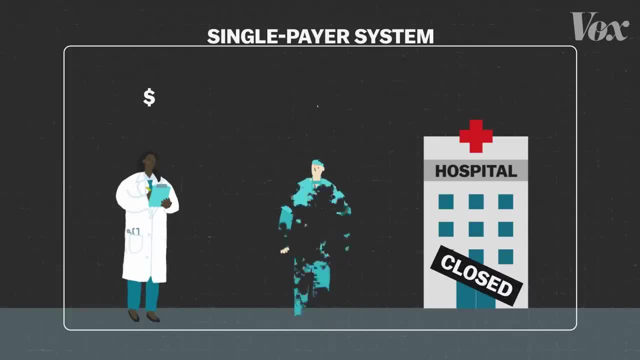 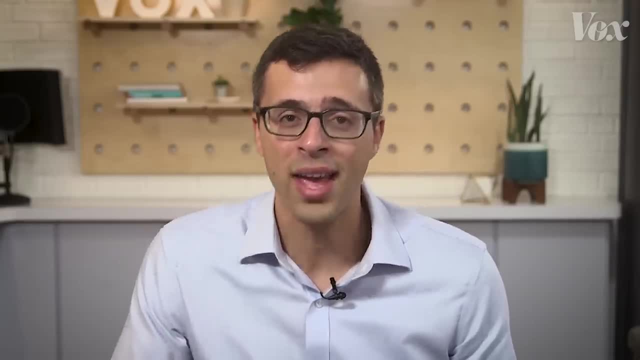 be paid less than they are right now. That might mean some of them close or some go out of business or some move. It would be really painful. One person's waste is another person's essential service or local hospital or their income, But then single payer it's not an. 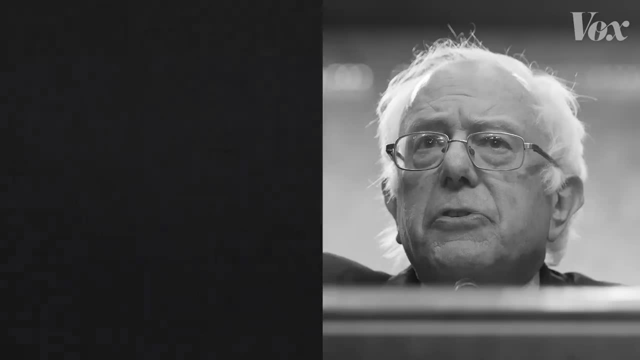 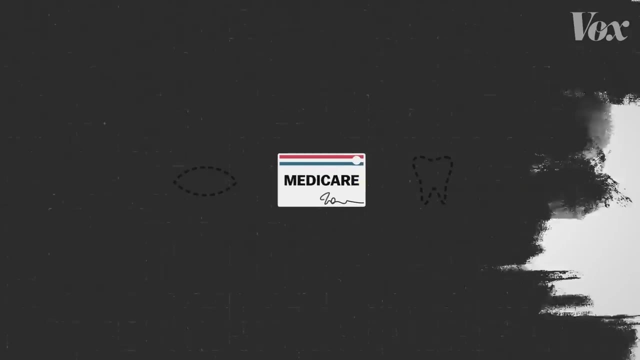 all or nothing choice. For instance, there's a really interesting section of Bernie Sanders' Medicare for All bill where he lays out this interim plan. It's a plan he wants while setting up his new single payer system And in that plan he expands Medicare to cover vision. 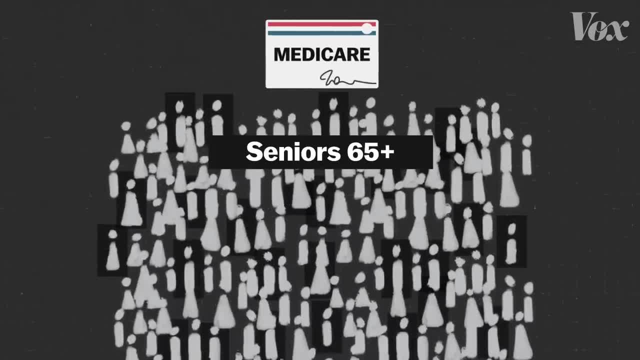 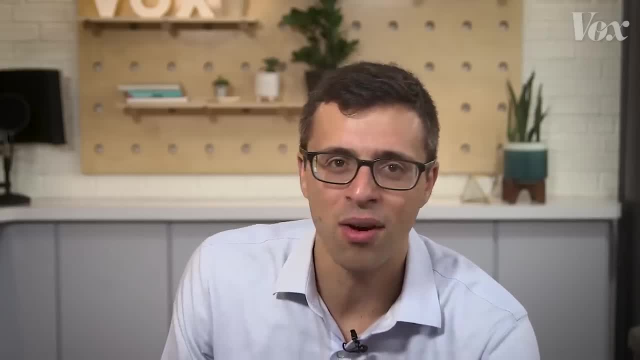 and dental, and he opens it to nearly everyone, not just people 65 and older. All kids go on Medicare automatically and most adults can buy in That plan on its own. it wouldn't get American health care spending far down overnight, but it would at least begin to. 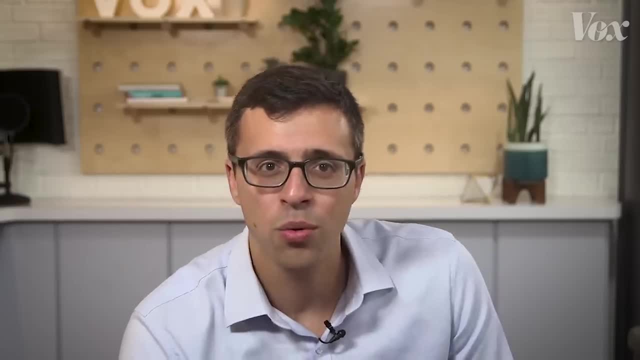 recognize what we already know and what most other countries already do: That health care is one of those things the government can do cheaper and better than the private sector. For more information, visit wwwFEMAgov. For more information, visit wwwFEMAgov. For more information, visit wwwFEMAgov.